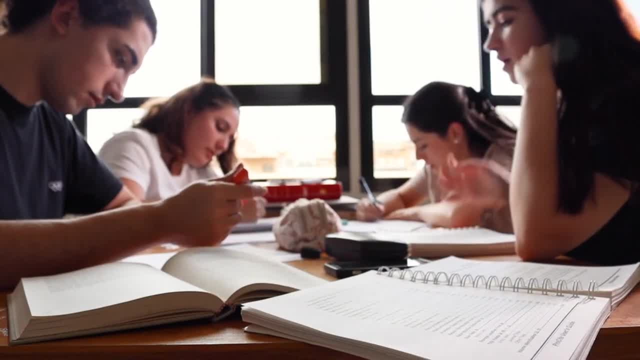 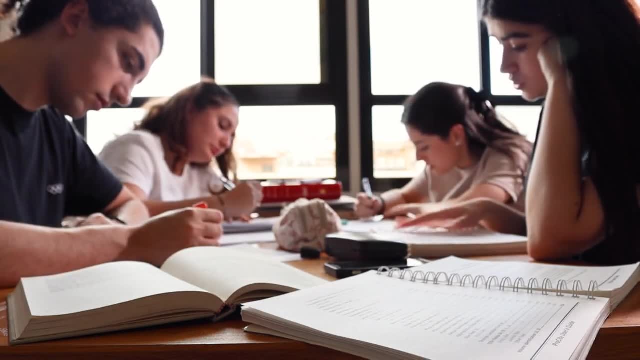 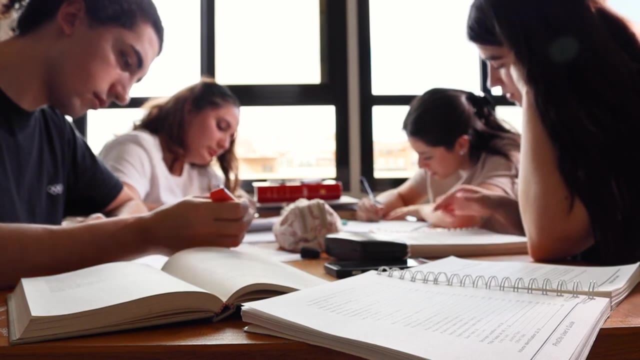 A main difference between neutrinos and other fermions such as the charge, leptons and the quarks is that neutrinos are the only known fermions that are electrically neutral. Hence the measurement of their electric charge cannot determine if the particle is a neutrino or an antineutrino. 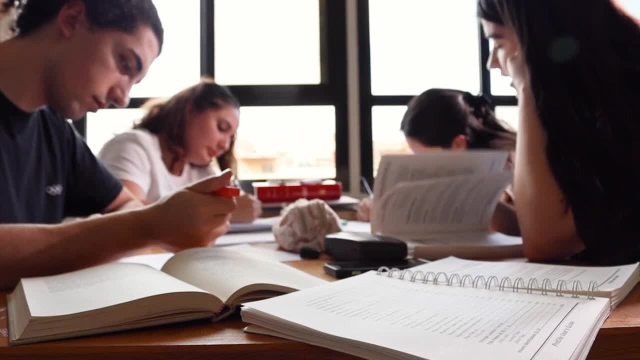 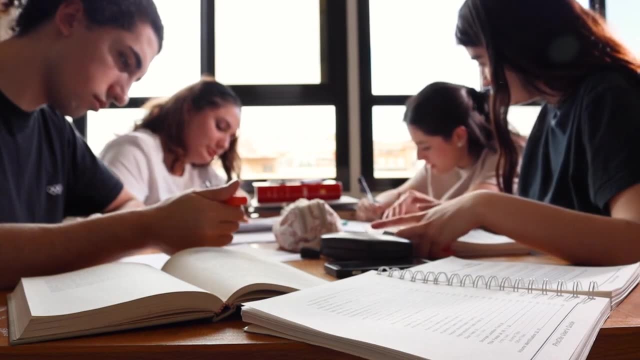 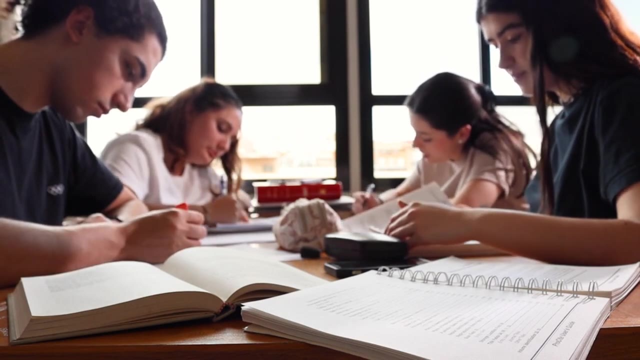 To distinguish a neutrino from an antineutrino, we must introduce the separate global lepton number. There is, however, no a priori reason for this global quantum number to be exactly conserved in nature. As a matter of fact, it is not known if the neutrino and antineutrino are indeed different particles or not. 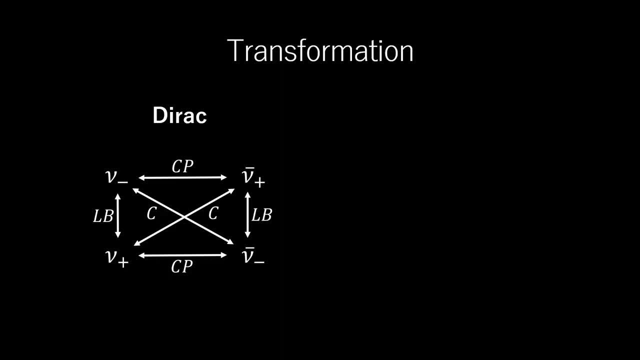 Let us consider the consequences of the Dirac nature of the neutrino field on the physical neutrinos and antineutrinos. Since we are assuming a Dirac field, we have a priori four degrees of freedom corresponding to the left-handed and right-handed chiral degrees. 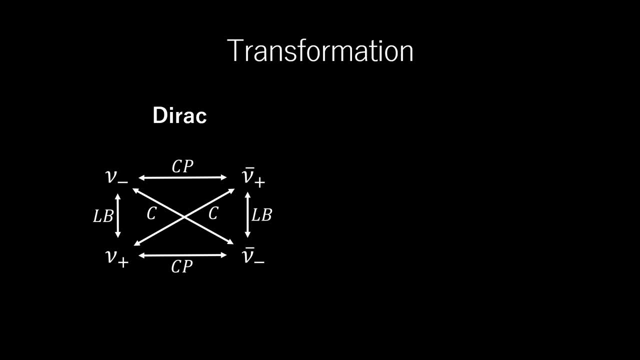 The four degrees of freedom correspond to chiral states with positive and negative energy solutions. In terms of helicity states, the four degrees of freedom correspond to two helicity states for each: neutrino and antineutrino. Considering the neutrino case, we label nu minus for the negative helicity state and nu plus for the positive helicity state. 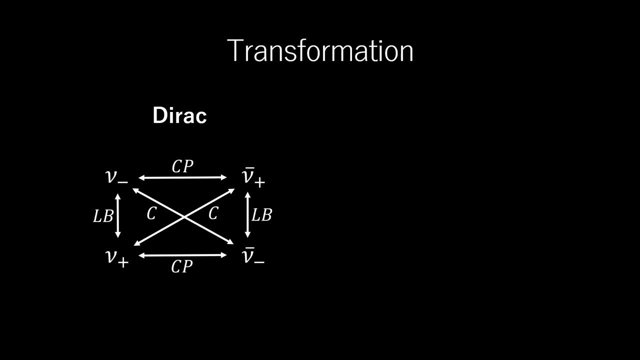 Similarly, the antineutrino can be in the nu bar minus or nu bar plus helicity states. We note that for a massive particle it is always possible to find a Lorentz booster. However, the boost does not alter the spin direction. 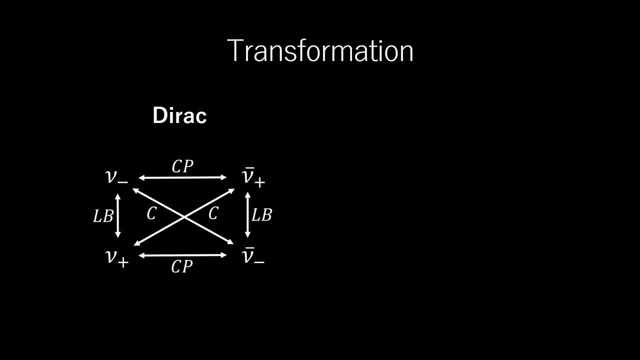 The two helicity states of a neutrino or of an antineutrino are therefore connected by such a Lorentz transformation. The charge conjugation operator C does not change the spin nor the momentum, and hence not the helicity. This can be expressed as the C transformation changing a particle into its antiparticle while leaving its helicity unchanged. 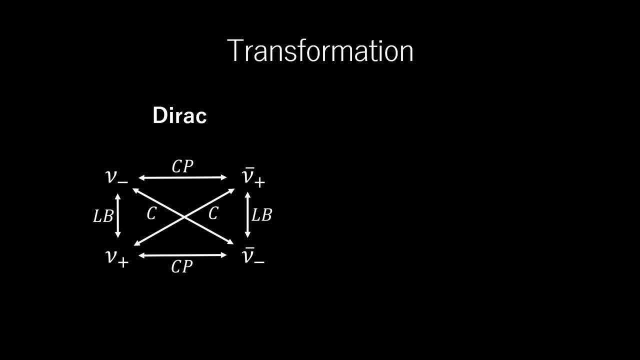 We should recall, neutrinos only participate in the weak interactions and with a pure V-A coupling. This means that the nu minus and nu bar plus are enhanced, while the nu plus and nu bar minus are highly suppressed. Hence the neutrino nu minus and antineutrino nu bar plus are connected C-P conjugates of one another. 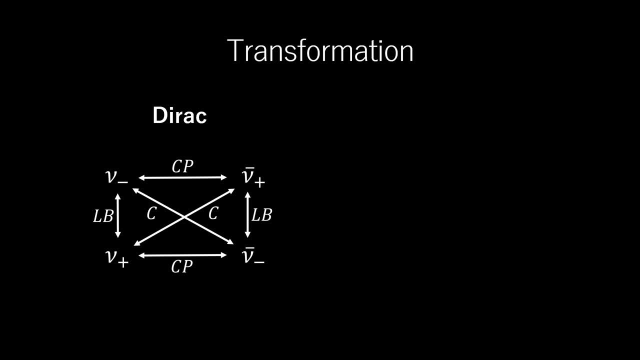 Similarly, the helicity states that are highly suppressed are evidently also C-P conjugates of one another. One can consider other scenarios. Could the neutrino, like the photon, be an eigenstate of the charge conjugation Majorana? neutrinos would possess only two independent states. 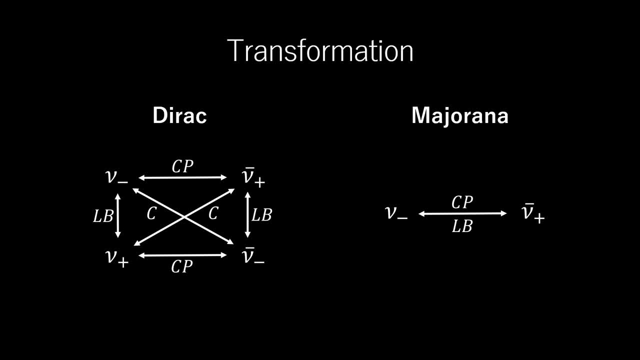 In the case where neutrinos are Majorana particles, the neutrino and the antineutrino C-P coupled states are also directly connected by a Lorentz boost. We have lost degrees of freedom, and the four degrees of freedom of the Dirac neutrinos are reduced to two degrees of freedom of the Majorana neutrinos. 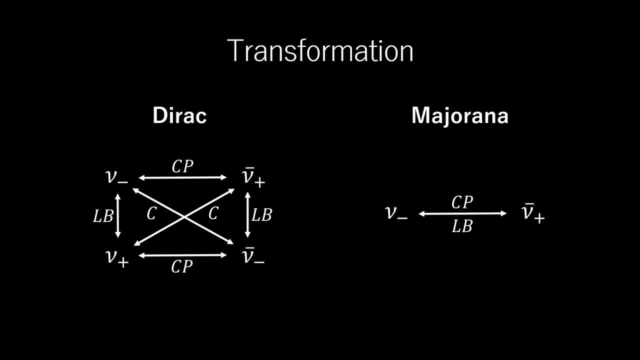 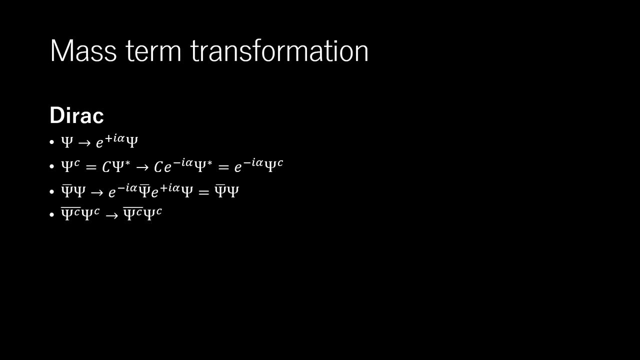 This is equivalent to stating that the known neutrinos in nature exist only in a left-handed chiral state. A global gauge transformation of our spinor implies, Hence the Dirac mass terms transforms under gauge transformation as, Therefore, they are invariant under our global gauge transformation. 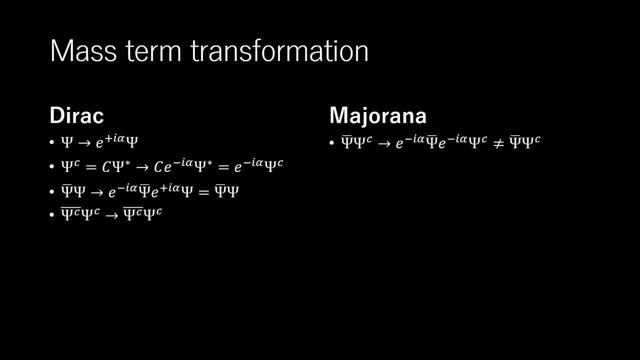 On the other hand, the Majorana mass terms lead to a gauge violation. This is interpreted as the violation of the lepton number. in our theory, The lepton number rises as the consequence of a U1 global symmetry, so there is no fundamental principle that allows us to state that this conservation should be exact. 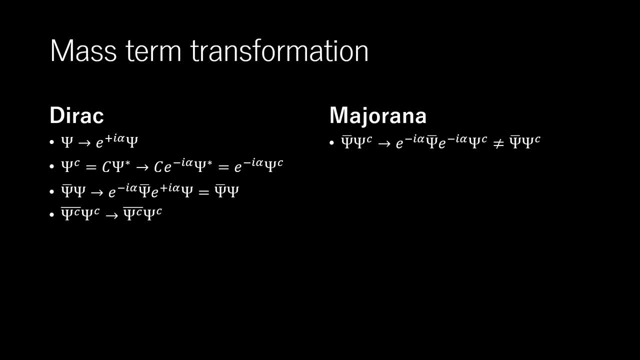 In the standard model, violation of the lepton number is not allowed and a lepton number violating Majorana mass term hence clearly represents physics beyond the standard model. 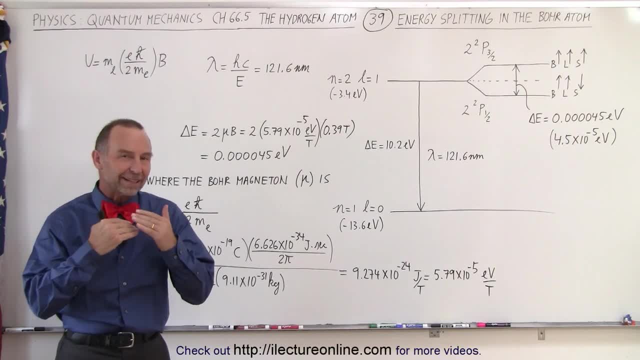 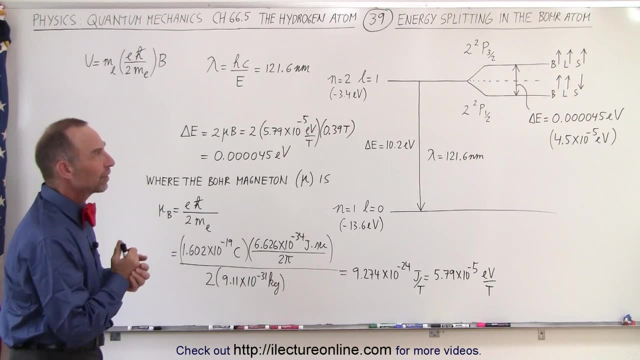 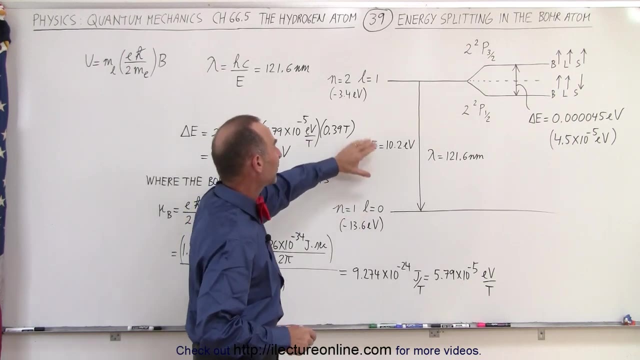 Welcome to our electron line. That slight splitting of the energies caused by the interaction between the electron spin and the orbital motion of the electron was first seen in the jump from the second level down to the first level in the Lyman series, where we have the energy difference of about 10.2 electron. 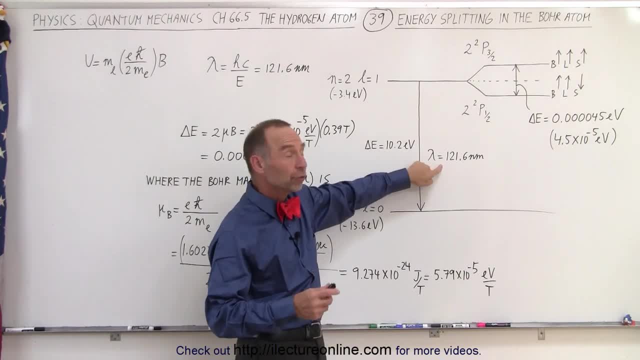 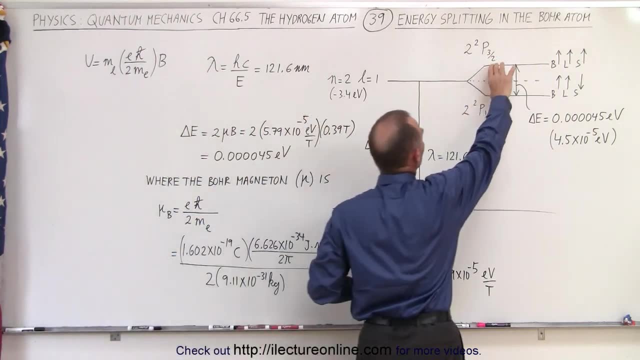 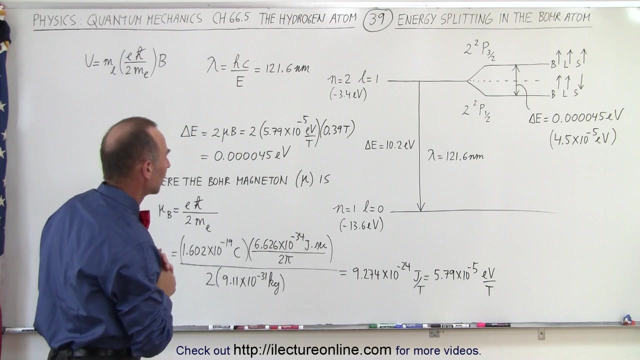 volts when we jump between these two levels, giving off a photon with a wavelength of about 121.6 nanometers. So again, what caused this slight splitting of the energy levels is the interaction between the spin of the electron and the magnetic field produced by the orbital motion of the electron. So if we calculate,